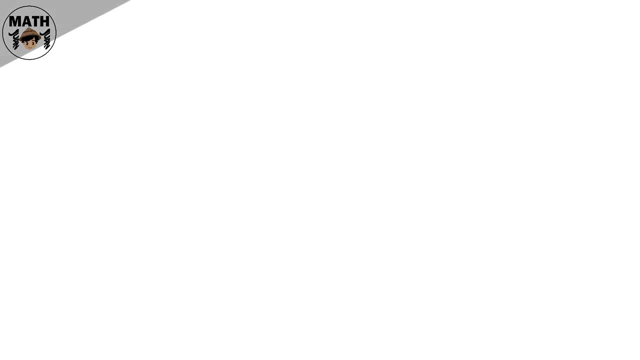 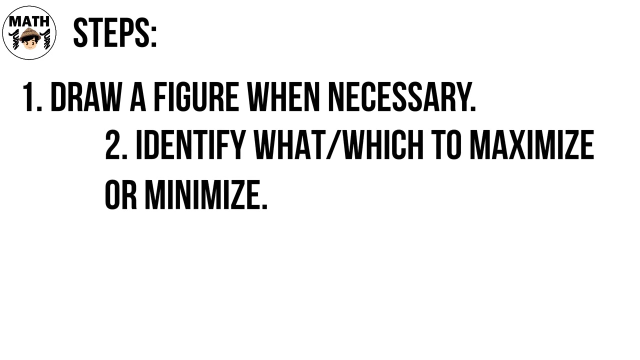 I'm looking for a maximum or a minimum value. Before we do that, we first have to develop the function that we're going to optimize. In developing the function, we can draw figures that are necessary to help us visualize the problem. Next is to identify what or which to 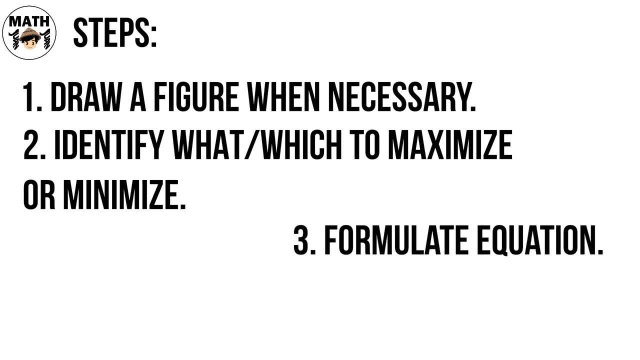 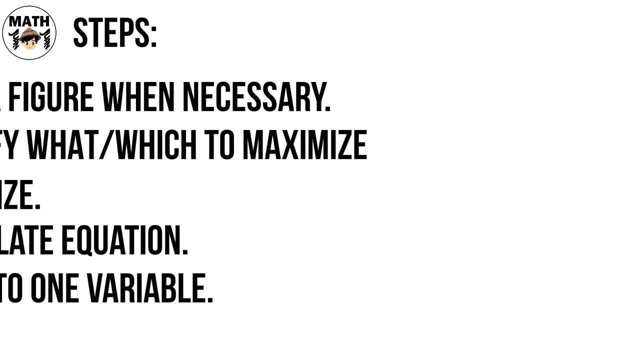 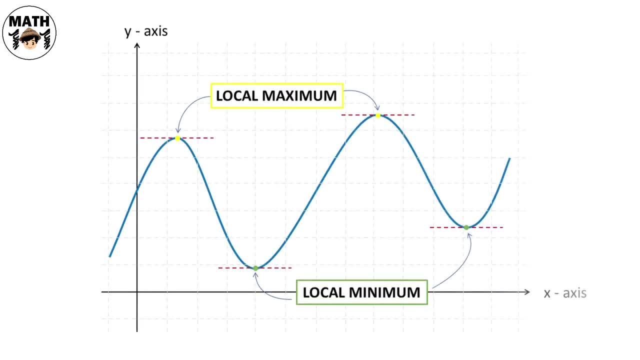 maximize or minimize. Then we formulate the equation, Then we write the equation, We reduce it to one variable before we can differentiate. And after reducing it to one variable, we differentiate and equate it to zero. Why do we equate it to zero? For a smoothly changing function, a maximum or minimum is. 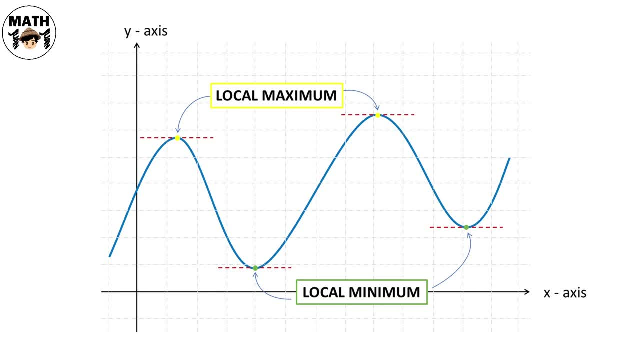 always where the function flattens out. Where does it flatten out? It flattens out to when the slope is zero, And we know that the first derivative gives us the slope of the function. So we equate the derivative to zero. After equating it to zero, we'll now solve for the 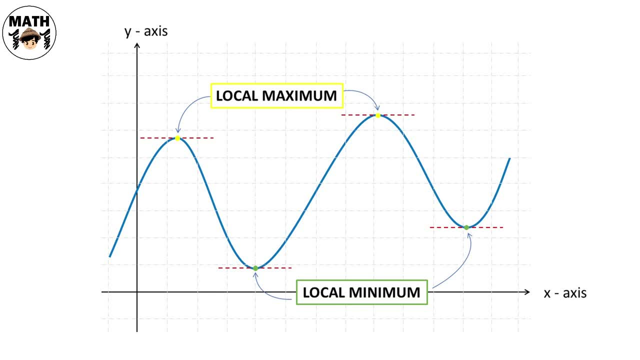 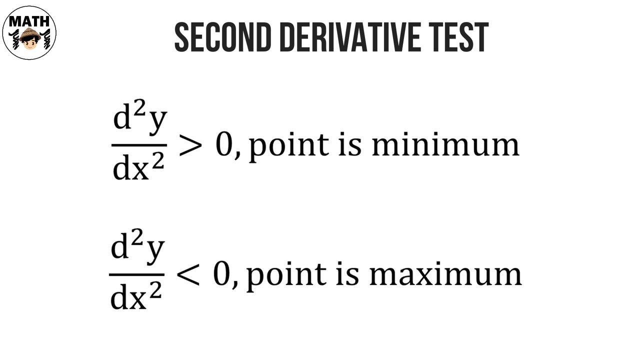 variables that are unknown in the problem. Sometimes, when we solve the equation, we get a lot of values. How do we know now which value we're looking for in the problem? We can use the second derivative test to determine whether the maximum point or minimum point. 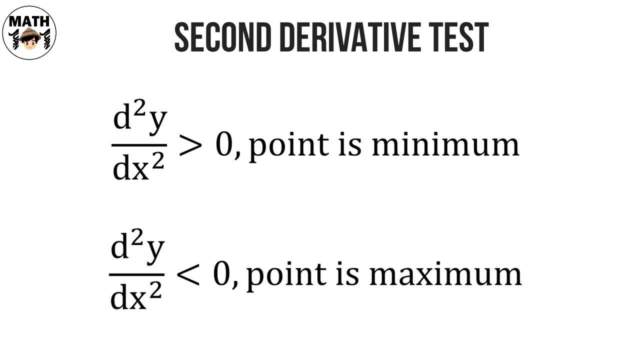 is what we got. So we solve for the second derivative. If it's greater than zero, the point is minimum, And if it's less than zero, the point is maximum. Now let us try to solve problems. Problem number one: find the maximum value of the product of two. 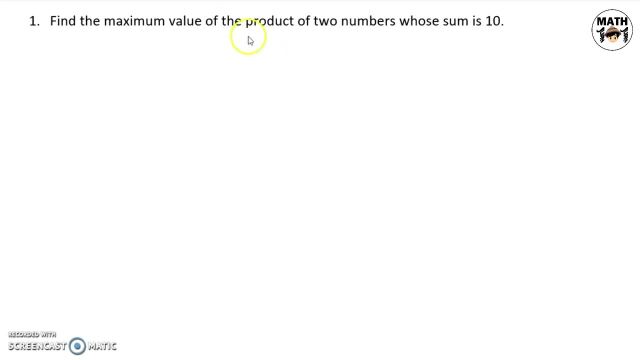 numbers whose sum is 10.. Our target to maximize here is the product, So we must formulate a function representing the product. Before we do that, let us first declare or represent the variables that we have in this problem. Let x and y be the numbers and p be their product. 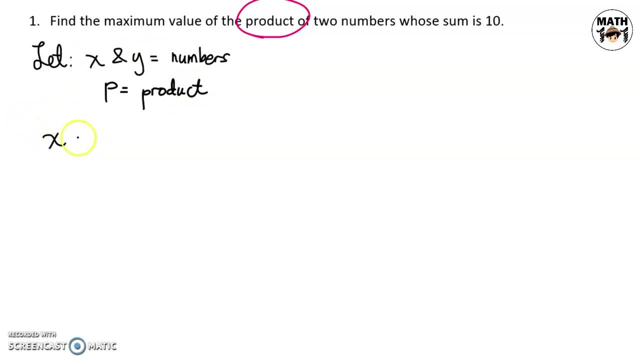 The sum of two numbers is 10.. x plus y is equal to 10. And their product, or p, is equal to xy. Before we differentiate, our function needs to be reduced to 10.. So let us first define the function. 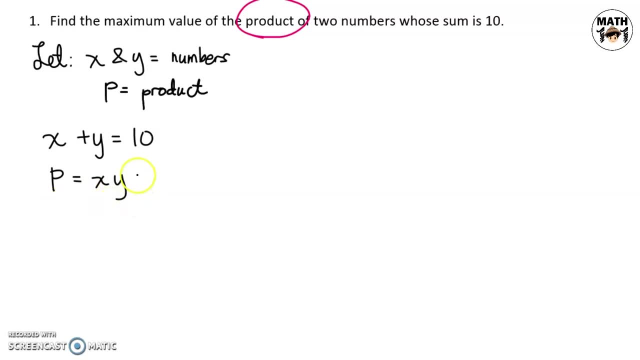 So let us first define the function. So let us first define the function. If y is the less than zero, greater than zero, then it's equal to 10 or greater than 2.. So when n is less than zero, there will be nothing special about n. 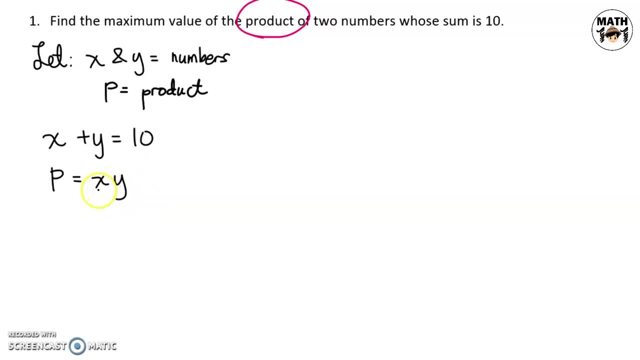 With this. we will just go ahead and say: let's rewrite it and transfer its value into one variable. So this will be how: x will be replaced by y. So, instead of x, y will be replaced by y. We replace x with y, if those Violator variables that are equal to 10, Tahiti variables. are equal to 1,, Ten and P, and these Violator variables will be replaced by y. If x equals 1 equal to 10 and P equals x minus Y, then it will be 1 equal to 10 or Ke. Surprisingly. 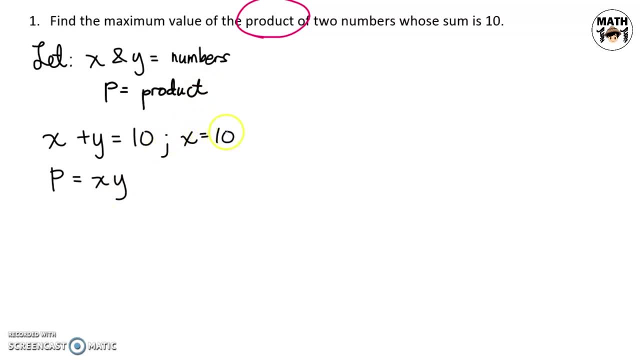 sh, f, t'n-y. So for P in constitution, this tomorrow, p is equal to 10 minus y multiplied by y, by y, 10y minus y squared. then let us now differentiate: derivative of p with respect to y is equal to derivative of 10y is 10. derivative of y squared is 2y. then let's equate this to: 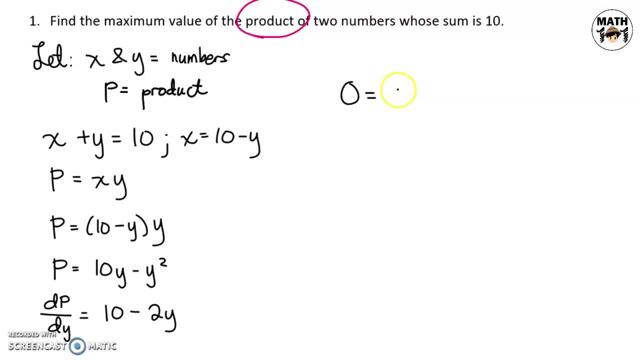 0, 0 is equal to 10 minus 2y. dipot natin sa kabila and we can now solve for y. divide both sides by 2, so therefore y is equal to 5, and to solve for x, ipalit lang natin to. 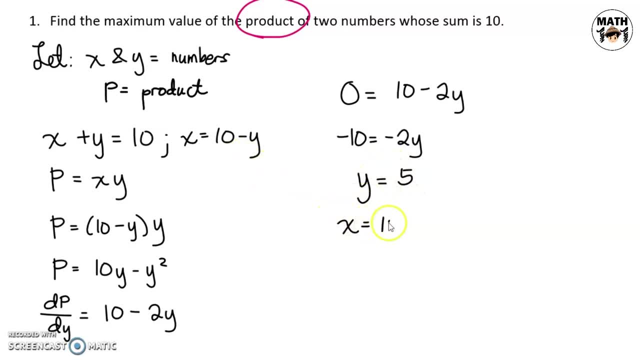 sa equation na to, x is equal to 10 minus y or 5, so x is equal to 5. now the two numbers are 5 and 5. ang hinahanap natin is the value of their product, so p is equal to 5 times 5, or that. 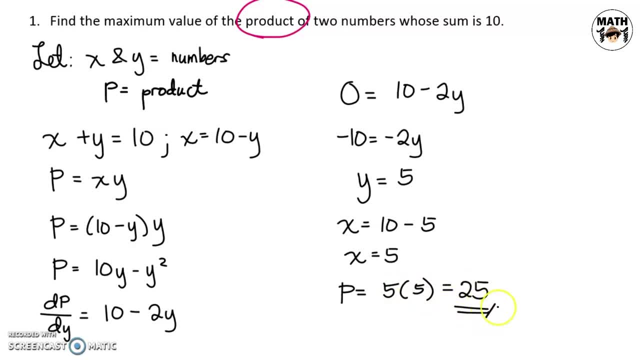 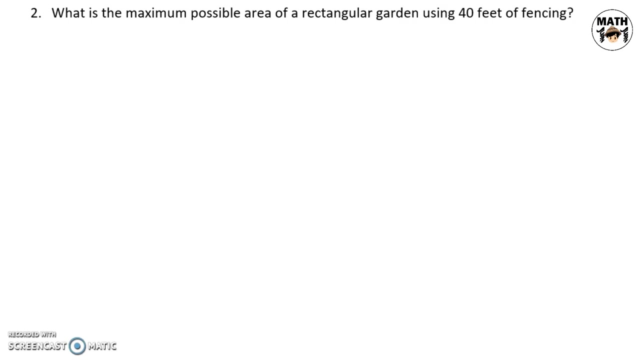 is equal to 25. so notice na for problems like this: kapag fix ang sum, yung dalawang numbers is just the half of that sum, or dapat lagi silang equal to get the maximum product. problem number two: what is the maximum possible area of rectangular garden using 40 feet of fencing? ang target? 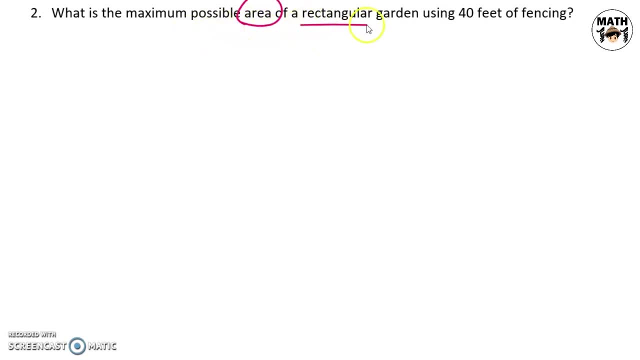 natin ma maximize is the area of a rectangular garden as much as possible. let us try to draw a figure for this. we have a rectangular garden, drawing their dimensions that represent the length as X and the width as y. so variable natin ngayon ay x, y and the area. we know that that is equal to the product of the 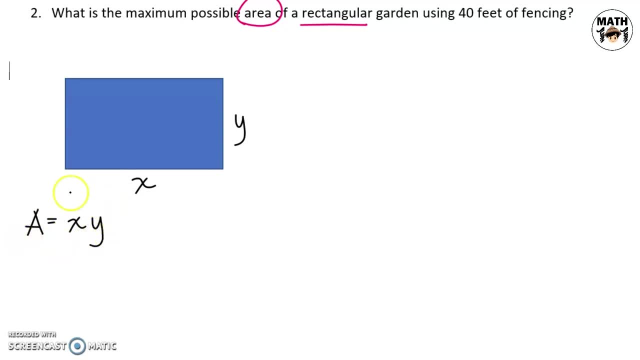 length and the width. before we differentiate, kailangan um we reduce, ric entender, one more variable nangyatana yung constrain natin dito. it is said that the fencing will be used is equal to 45, and ba yung 40 feet na yun, So yung 40 feet na yun. imagine if a fence ito, ito, ito, tsaka ito, So. 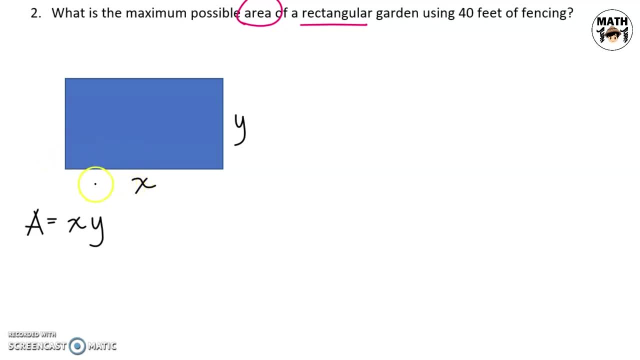 yung 40 feet na yun. that will be the perimeter nung ating rectangular garden. So 40 is equal to the sum of the sides, or that is just 2x plus 2y. Dividing this whole equation by 2, we can arrive. 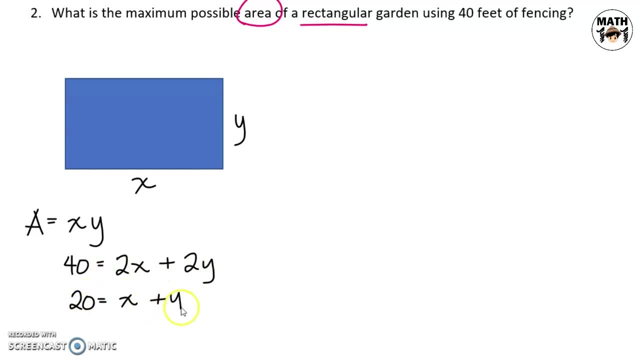 at 20 equals x plus y. So pwede nating isulat si y in terms of x or si x in terms of y, Palitan na lang. ulit natin yung x in terms of y and we'll have x equals 20 minus y. Palit natin to dun sa. 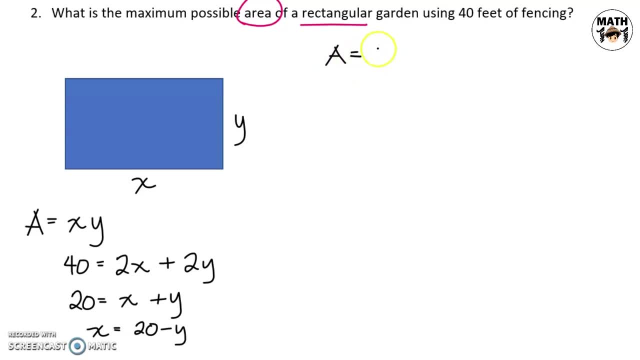 ating equation, We'll have a equals 20 minus y multiplied by y. Expand this and we have the area as 20y minus y squared. Let's differentiate now, since na-reduce na natin to in one variable: Derivative of a with respect to y is equal to 20 minus derivative of y squared is 2y. 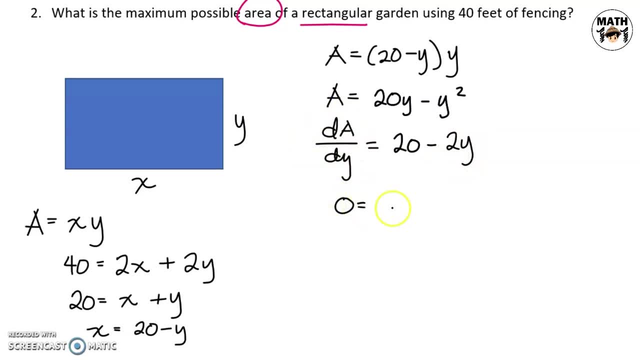 Then let's equate this to 0.. 0 equals 20 minus 2y and we'll get negative. 20 equals negative 2y. Therefore y is equal to 10.. And solving for x or ating length, we have 20 minus y, So x is equal to 10.. 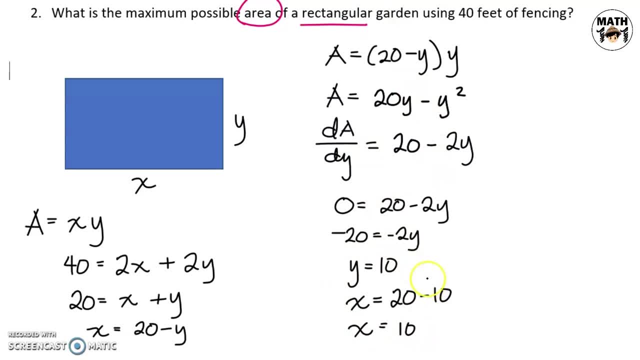 Notice yung similarity nung problem na to dun sa ating previous problem. Ang nangyari is yung sum is parang na-fix sa 20.. So we know na para ma-maximize yung product dapat maging equal yung dalawang number And, as we can see here, equal yung ating length and width. 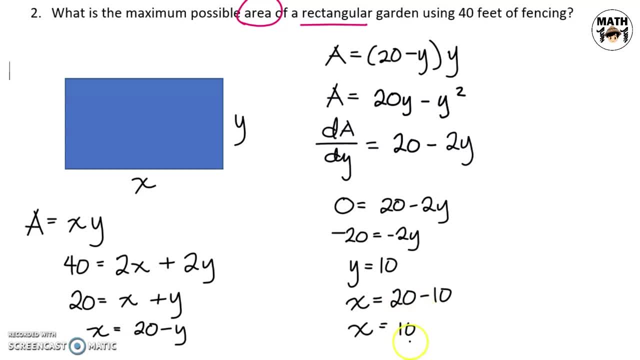 So, given a perimeter, we know that the maximum area will happen if the sides are equal or kapag sila ay naging square. So the maximum possible area for this is just the product of the sides 10 times 10.. Ang unit natin dyan ay feet.